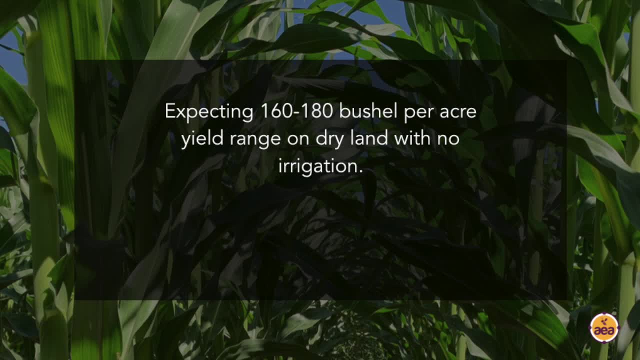 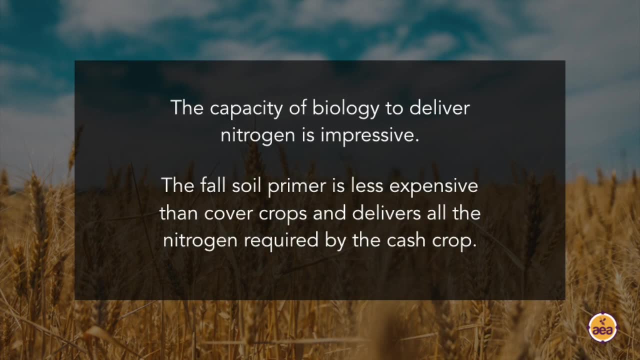 impressive. What I'm really impressed by is the capacity of biology to deliver nitrogen. A farmer made the comment. he said I can use the fall soil primer less expensively than growing a cover crop to deliver all of my nitrogen requirements. There was no other nitrogen. 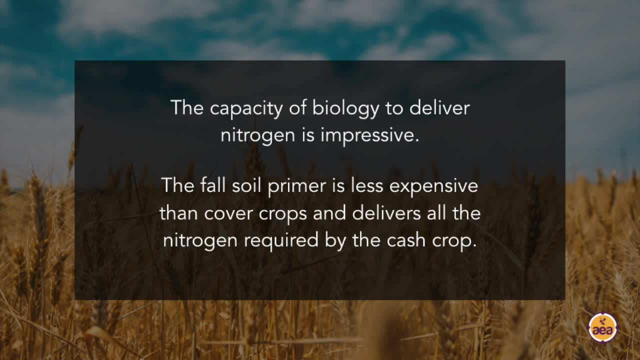 requirement other than the nitrogen that was released from biology and fixed from the air and made available to the crop. So there have been a lot of conversations in the regenerative agriculture space by growers and agronomists who've been speaking about the capacity of biology. 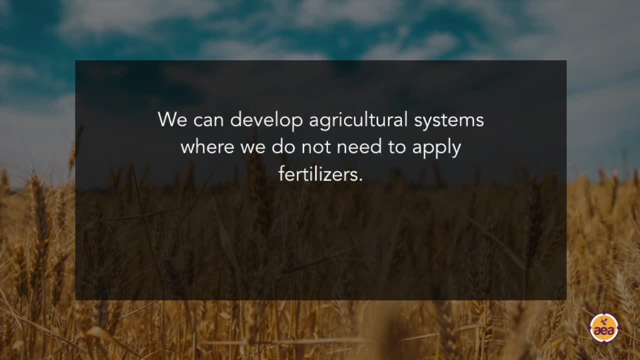 to deliver nutrients And the idea that we can develop agricultural models and systems where we do not need to apply fertilizers and where we don't need to apply nitrogen and phosphorus and potassium, because biology can fix nitrogen from the air and can release phosphorus and potassium from the locked. 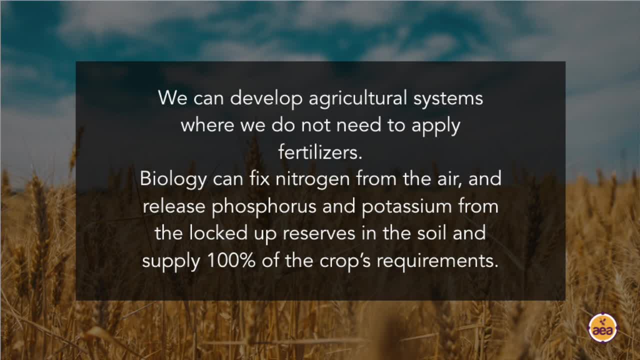 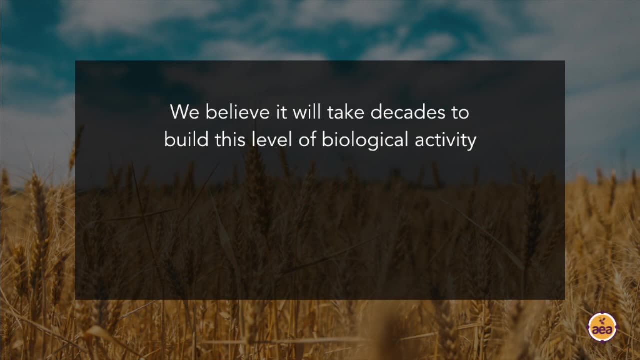 up reserves in the soil and supply 100% of our crops requirements. There are many examples where this has actually been demonstrated to be true for extended periods of time on a number of different farms, And often the idea is that it takes a lot of time to get to this level of productivity and biological activity. 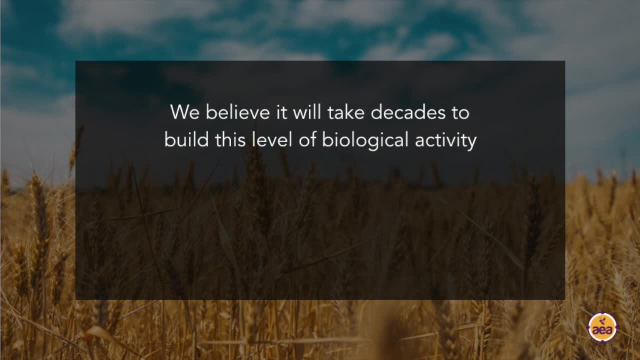 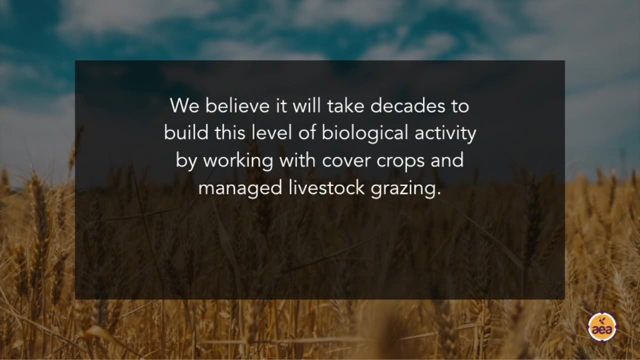 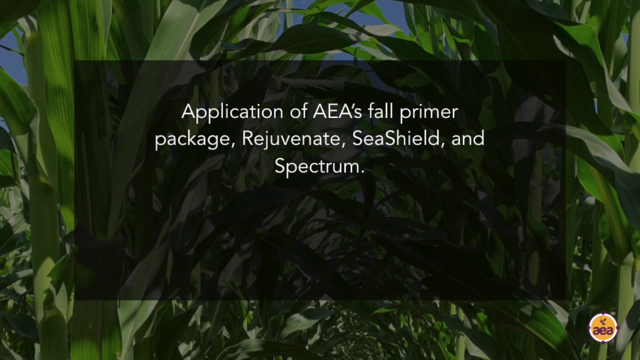 It'll take a decade or a couple of decades of working with cover crops and rotational grazing of livestock etc. to achieve soil biology to that level of performance. But this grower didn't do any of those things. He only applied Rejuvenate and Spectrum and Seashield our fall soil primers. 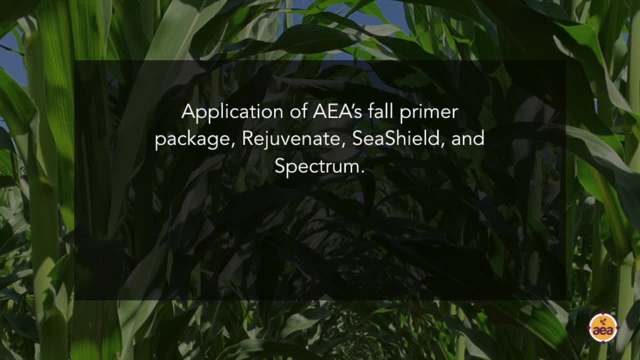 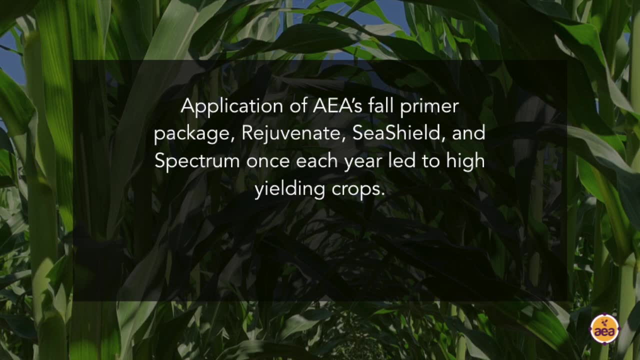 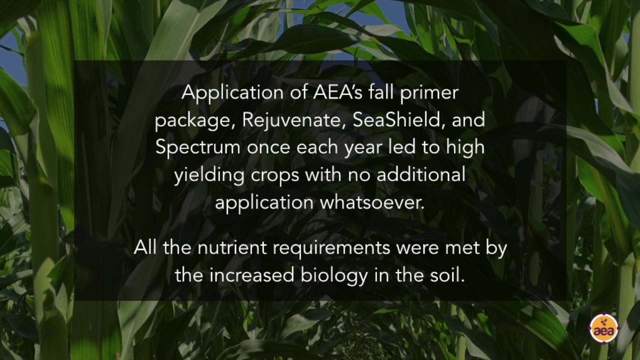 fall soil primer package, the fall before planting his crop- and he was able to achieve those types of results. In fact, he was able to achieve those results after only three applications. There's been all these theoretical conversations about what is possible and what can be achieved. 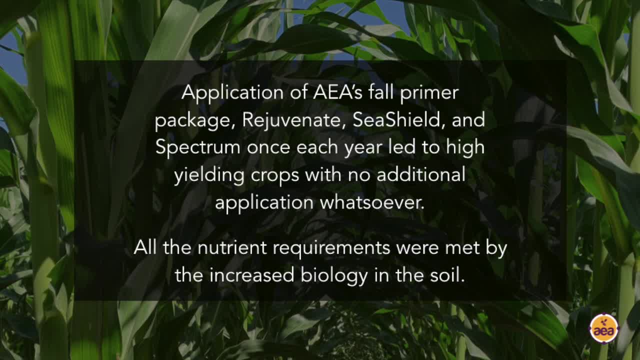 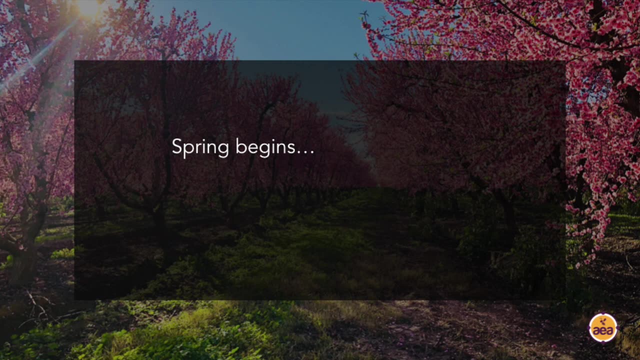 by having an optimum biological population. But what I'm excited about so much is the idea that we can accomplish those types of results in a matter of a year or two or three, and not measured in decades, As farmers being connected to the cycles of the planet and harsh winter months. 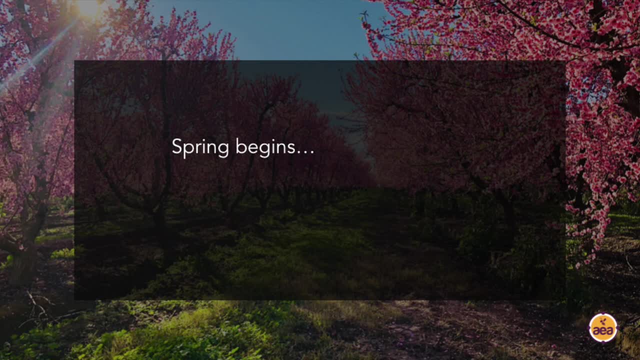 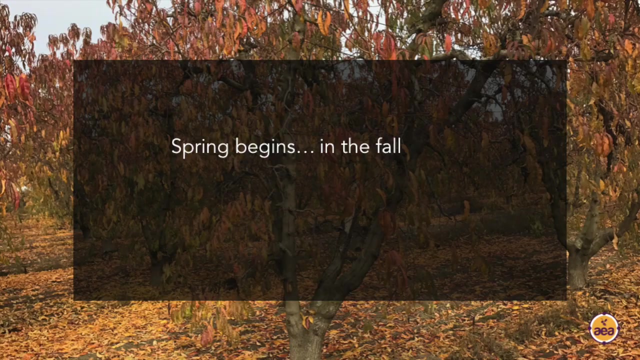 the rebirth of plants in the spring. it is usual and common for us to think about the season beginning in the spring, But in reality, when we start thinking about developing our soil microbial populations, our season doesn't begin in the spring. Our season needs to begin in the fall. 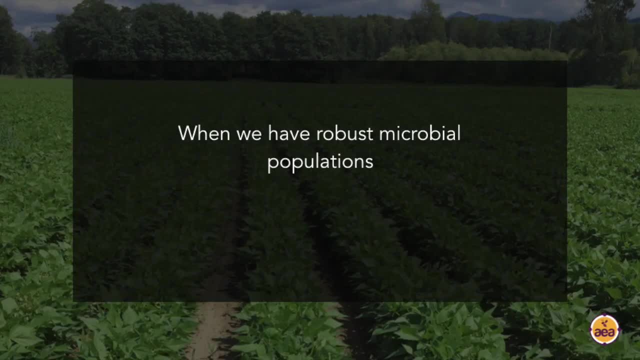 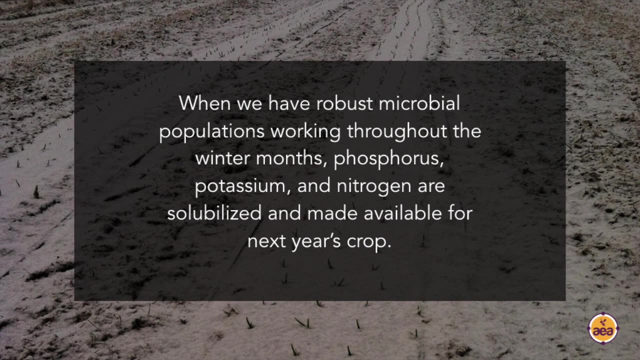 Because when we have robust microbial populations working in the soil throughout the winter months, they have the capacity to release a lot of nutrients, solubilize phosphorus, solubilize potassium and fix nitrogen and make it available for next year's crop. 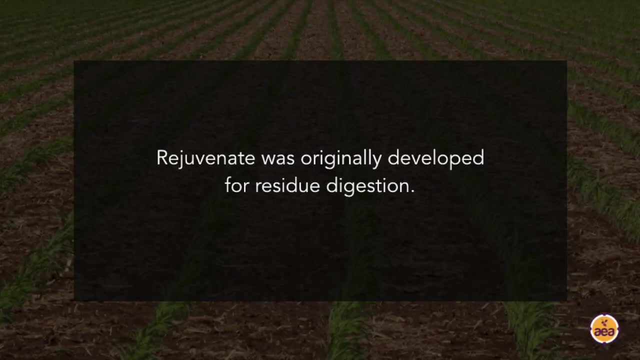 We originally developed Rejuvenate to increase residue digestion in the fall, so that we get rid of the residue, we remove disease carryover and so that we have very strong disease-suppressive soils the following year to suppress potential pathogens from causing an infection. 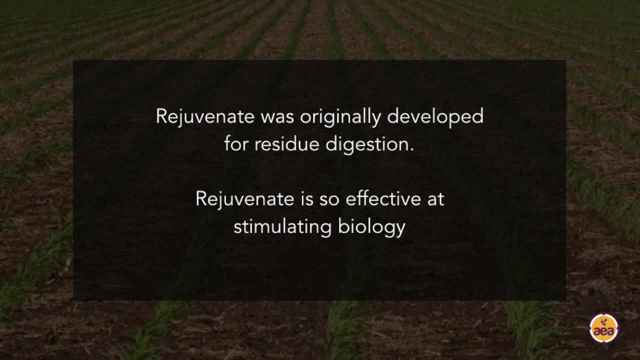 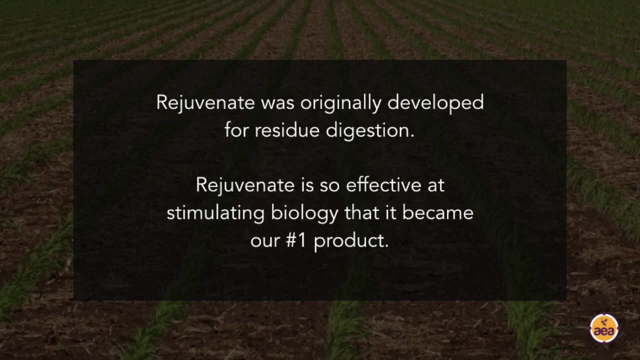 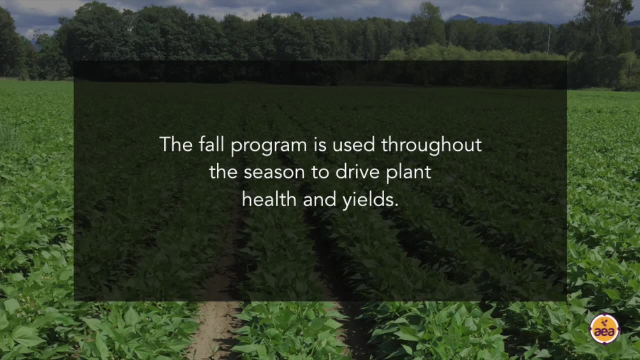 And Rejuvenate was so effective at stimulating biology to have all these effects on the soil environment that it's become our number one product. It's used by growers of every different type of crop and it's become so widely used that growers today are also using it during the growing season. 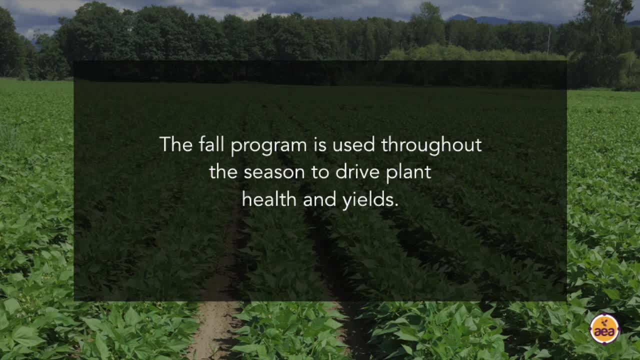 They're applying it in the furrow at planting, They're putting it in irrigation, They're putting it in irrigation systems and using it throughout the season And it certainly is providing a strong benefit and a strong crop response when used in these environments. 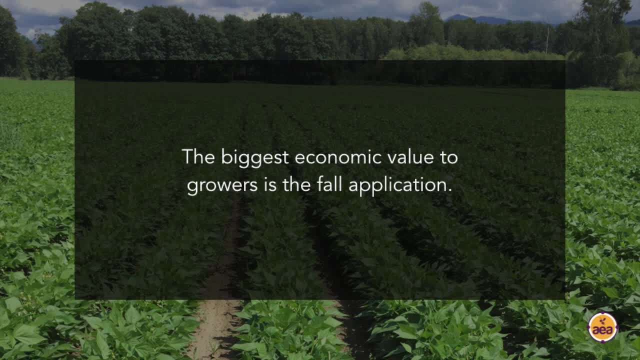 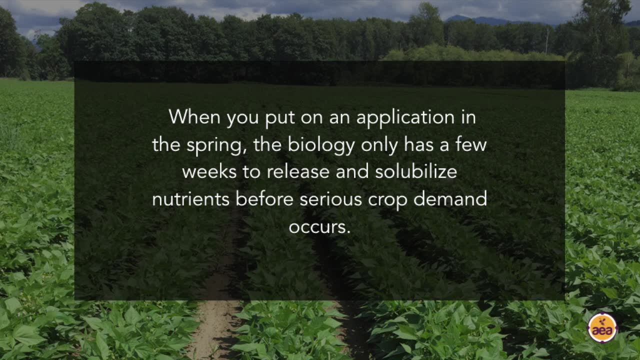 But still the biggest economic value that it provides to growers is the fall application, Because when you put on an application in the spring- let's say you put it on in the furrow at planting- the biology that is added in the soil only has a period of a few weeks. 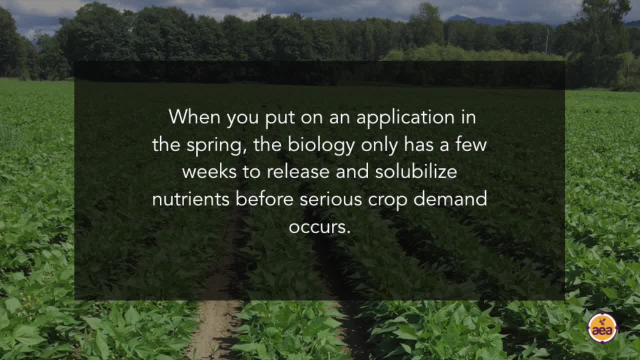 to a month or so in which it can release and solubilize nutrients before we start getting to a point of very serious crop demand and the crop begins pulling a lot of nutrients out of the soil profile When we apply the fall primer in the fall. 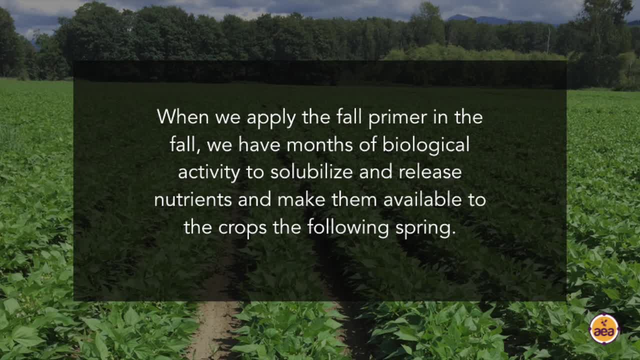 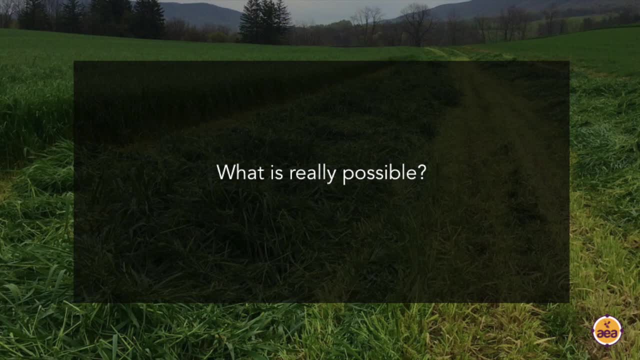 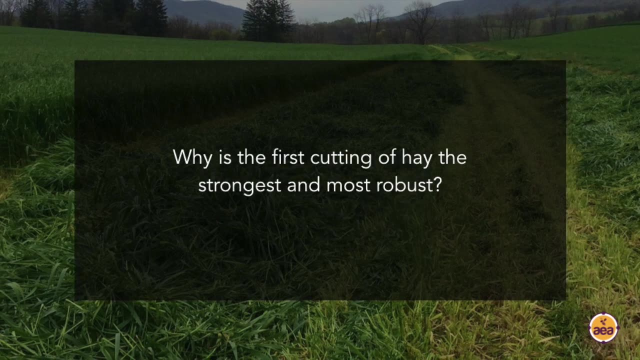 we now have months of biological activity to solubilize and release nutrients and make them available to the crop the following spring. You know I'll use a hay crop as an example of what really is possible. We've become used to the idea that the first cutting of hay should be the strongest and the most robust. 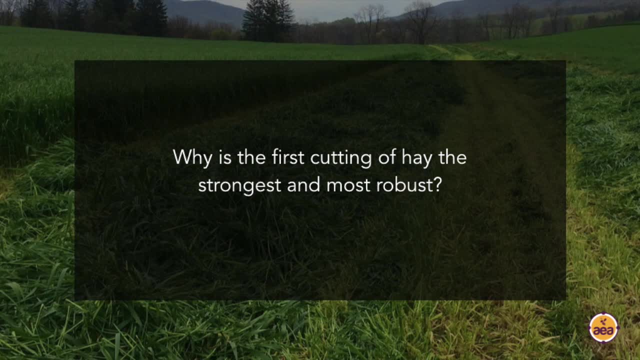 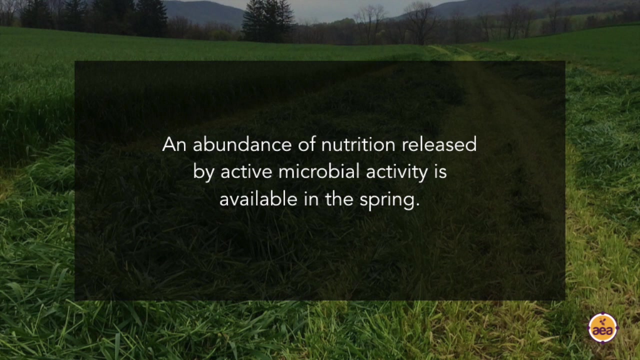 bust in the spring, And this is due to a couple of different reasons. It's partially due to moisture- We have very good moisture levels in the spring- But it is also due to an abundance of microbially active nutrition, where we had all the nutrients that were released through the winter months. 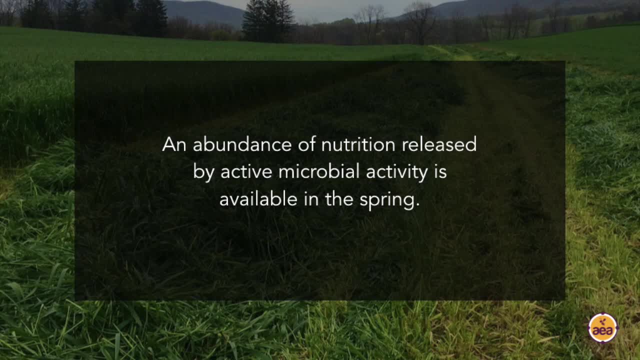 solubilized. And now the first growth of alfalfa in the spring. the first growth of hand in the spring has this abundant nutrient supply from soil biology, So we get very robust growth. And then the second cutting is significantly less. The third cutting is even less. The fourth cutting 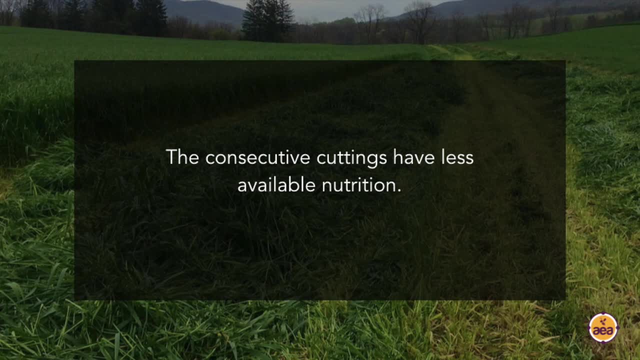 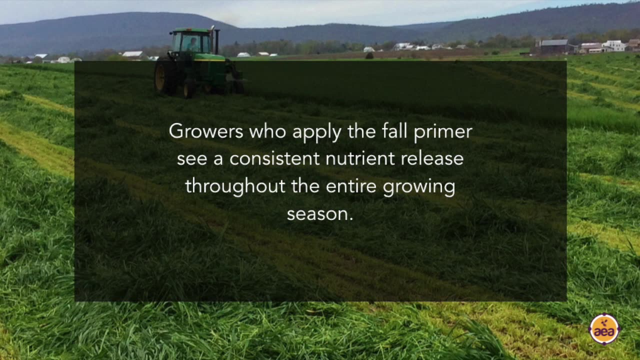 is even less And it tapers off throughout the entire growing season, And this varies, of course, depending on the environment and which region of the country we're speaking about, But we have worked with growers who put on the fall primer in the fall and produced not just. 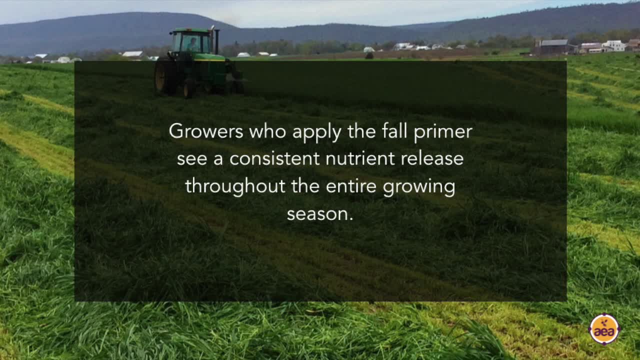 a tremendous nutrient release from soil biology, but a consistent nutrient release not only during the winter months but also the following summer, so that there was no drop-off in yield in later cuttings. In fact, one of the growers that we worked with has produced higher yields in the 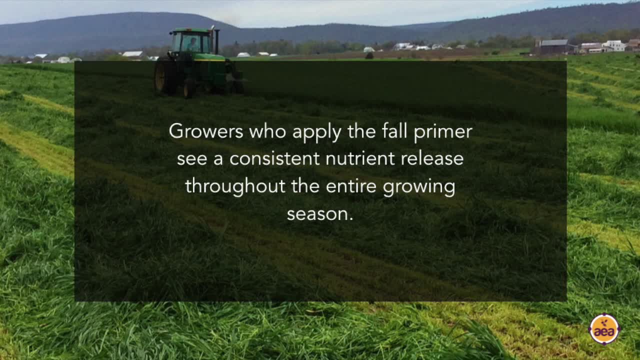 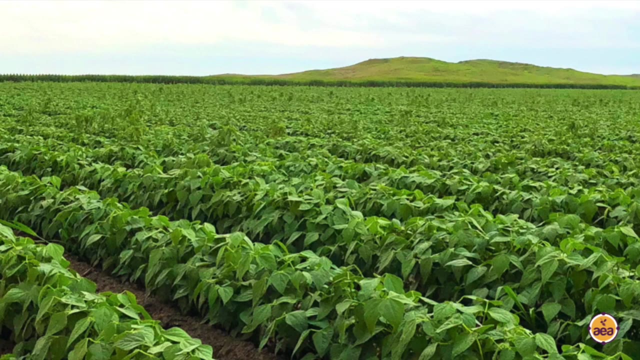 second and third and fourth cutting he did. in the first cutting The yields constantly improved throughout the entire year, both in terms of actual yield and in terms of forage quality as well. Imagine what can be delivered to a corn crop or a soybean crop when you have such robust biology that they 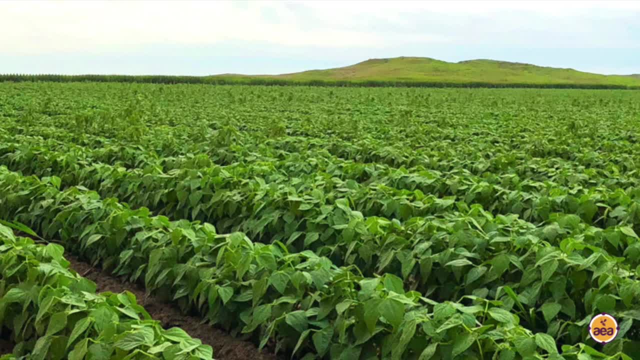 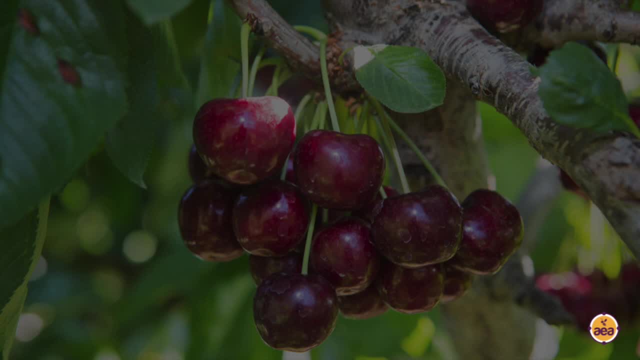 can actually supply 100% of the crop's nutrient demands when you get to the grain fill period or when you get- and the same is true of tree fruit and nuts and vegetable crops as well. Imagine what would happen and how plants would behave differently if the soil biology was able. 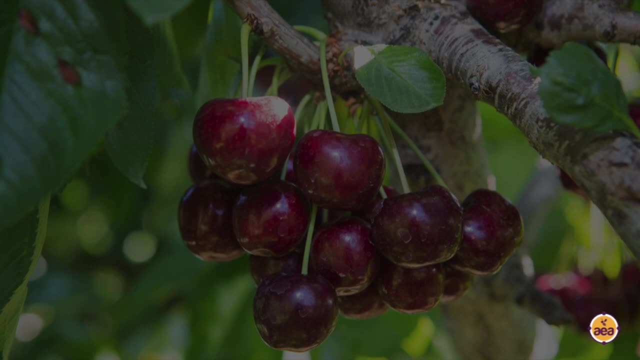 to supply 100% of the crop's nutritional requirements. We know that this can happen depending on the soil geology. Of course, you have to have a soil profile that has the presence of potassium and phosphorus that can be released. We can supply 100% of a crop's nutritional